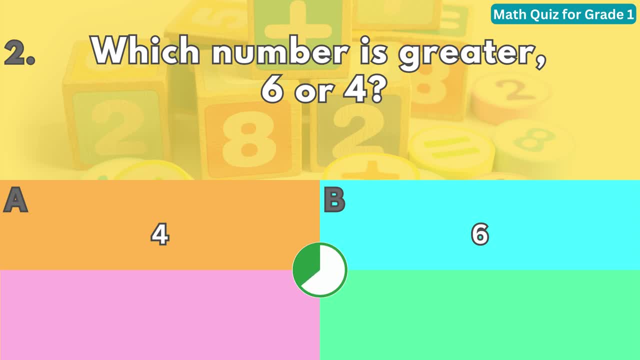 The correct answer is letter B. To determine which number is greater, you can compare them. When we have 6 objects and 4 objects, 6 is more than 4.. Question number three: What is the value of 2 times 3?? 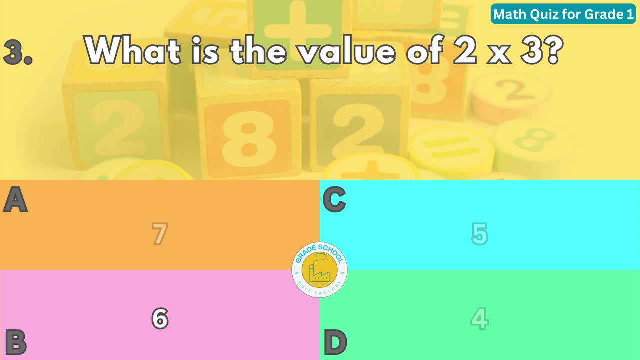 The correct answer is letter B. To multiply 2 by 3, we can add 2, 3 times 2 plus 2 plus 2 equals 6.. So 2 times 3 equals 6.. Question number four: How many sides does a triangle have? 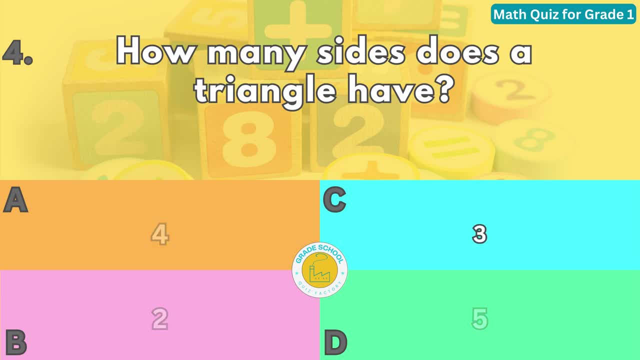 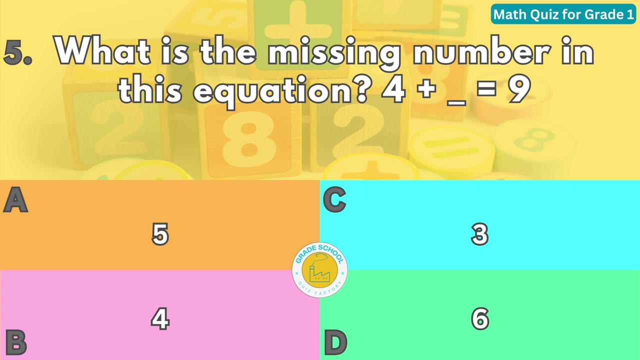 The correct answer is letter C. A triangle has three sides. If you look at a triangle, you will see that it has three straight lines and three corners. Moving on to question number five, What is the missing number in this equation? 4 plus blank equals 9.. 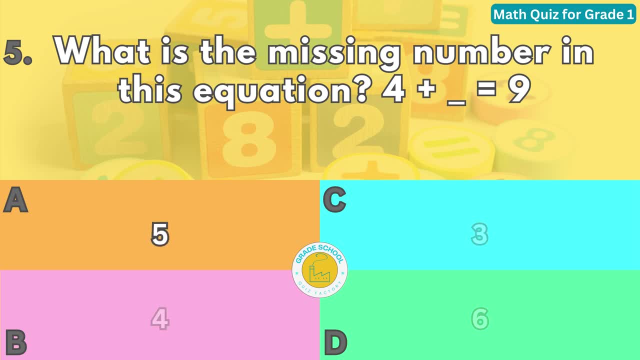 The correct answer is letter A. To find the missing number we need to subtract 4 from both sides of the equation. 4 plus blank equals 9. becomes blank equals 9 minus 4.. Blank equals 5.. So the missing number is 5.. 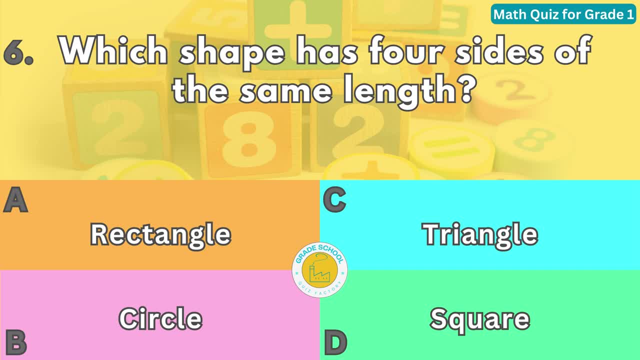 Question number six: Which shape has four sides of the same length? The correct answer is letter D. A square has four sides of the same length. Look at the sides of a square and you will notice that they are all equal in length. 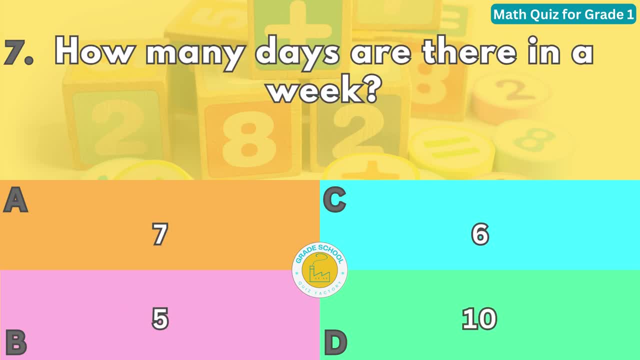 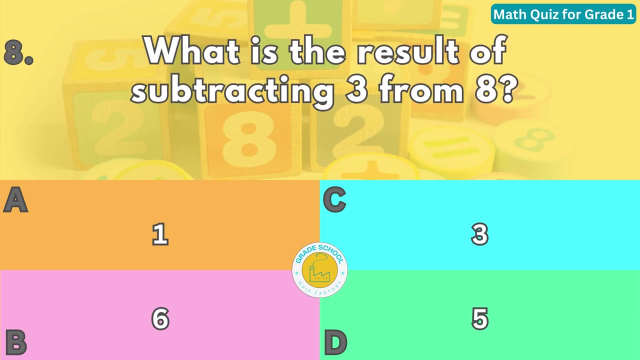 Question number seven: How many days are there in a week? The correct answer is letter A. There are seven days in a week named Sunday, Monday, Tuesday, Wednesday, Thursday, Friday and Saturday. Question number eight: What is the result of subtracting 3 from 8?? 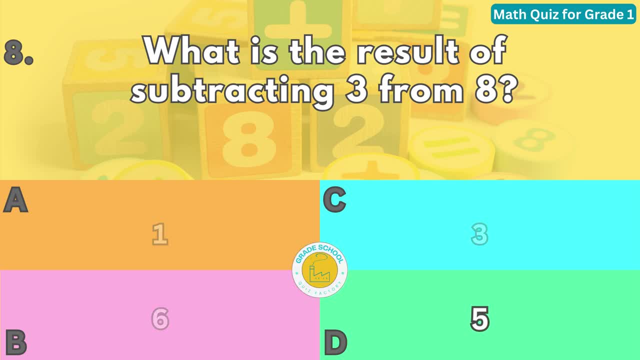 The correct answer is letter D. To find the result of subtracting 3 from 8, you need to take away 3 from 8.. Imagine you have eight cookies and you eat three of them. You will have five cookies remaining. Question number nine: